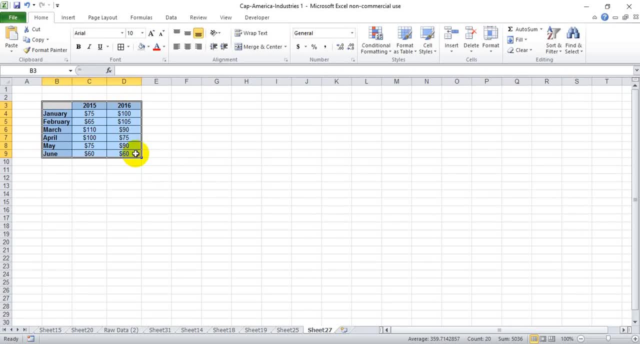 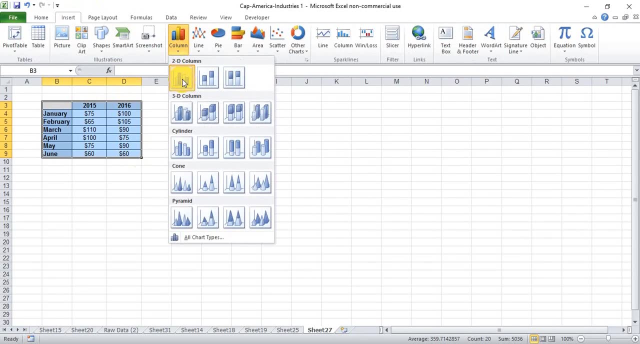 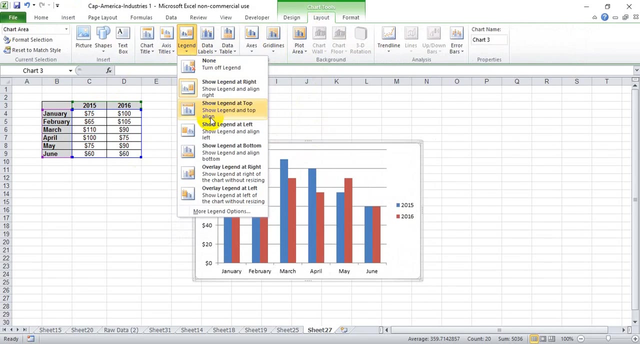 sales figures for year 2015 and 2016 and we're going to go ahead and put it in a standard 2d clustered column format, which is the first option in the top left, and we see chart type. that is fairly common but we're going to tweak. 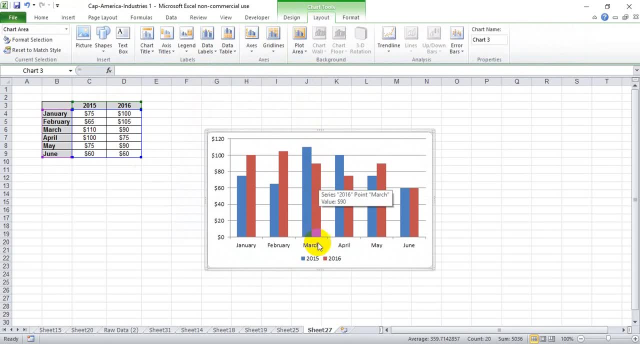 it a little bit to make it look a little more interesting. So we want 2015 to kind of take a backseat to the most current data, but we want it to create almost a container so we can show how much more or less we're showing in the current 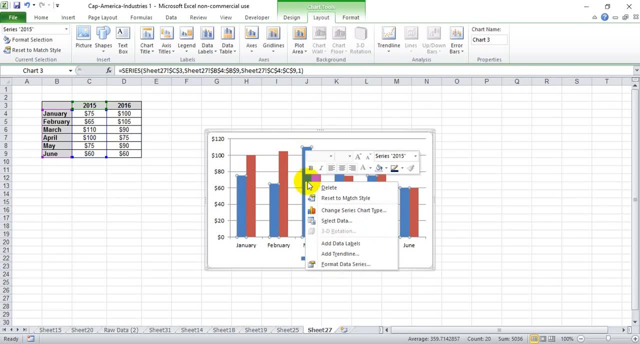 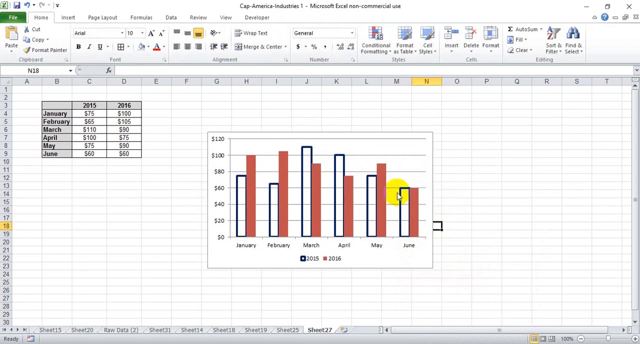 year. So we're going to go ahead and do is select the older of the two years and remove the fill from that year. However, we're going to give it a pretty large outline, say weight 3- I think looks pretty decent. and then we're going to go into our data set and format the data. 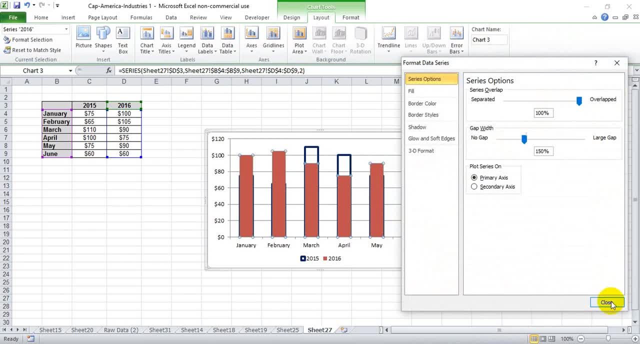 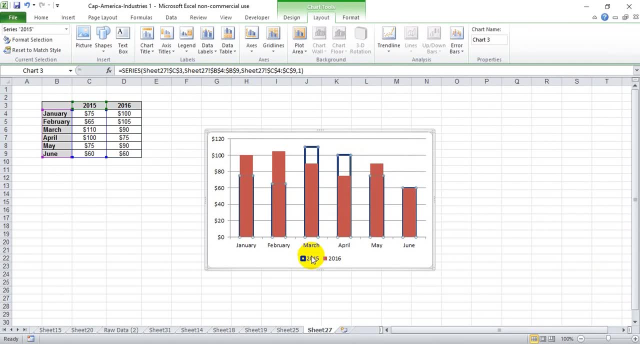 series and we're going to overlap it to a hundred percent and close our data set here. We're going to deselect everything, but then we're going to go back and touch one of the 2015 columns so that all of them are selected, and we're going to go. 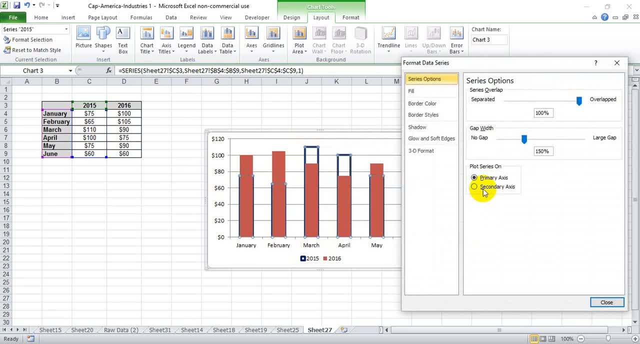 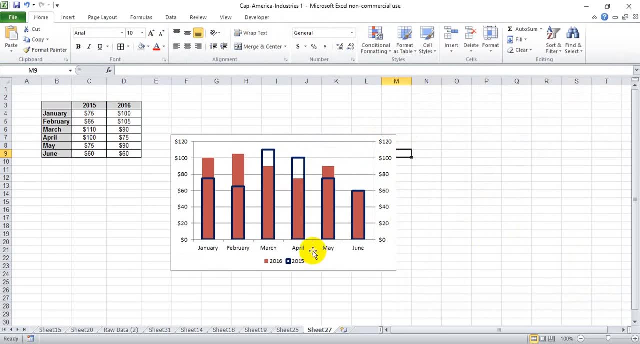 ahead and right-click and format data series again and we're going to go ahead and put that on the secondary access so that it comes to the forefront. So right now we can see the 2015 sales data is still present, but it's kind of taking a backseat to the more pronounced 2016. 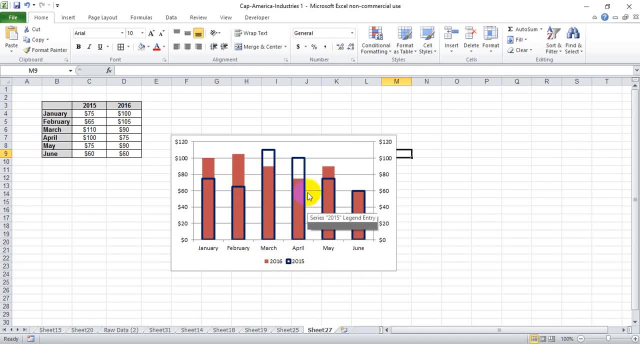 data and if you think that it would look more appropriate if this was a smaller border- I could see the argument there- or maybe a more subtle color or to change the transparency, but I think it's a really cool way to show year-over-year sales so that you can show the performance. 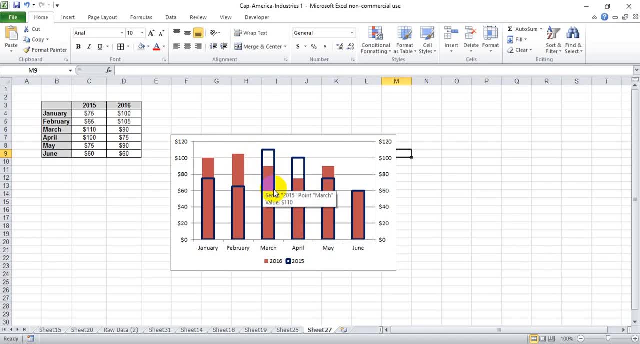 improvement or decline from the previous year. Thanks a lot for watching. I hope this helps.